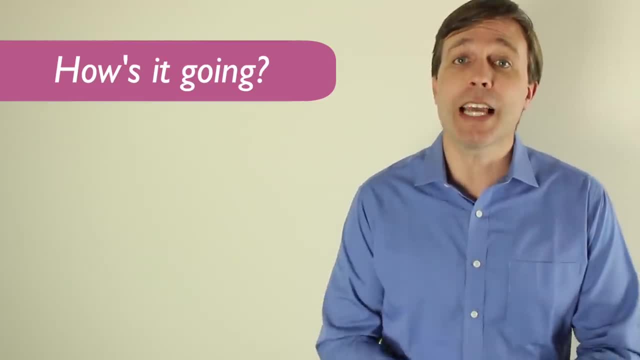 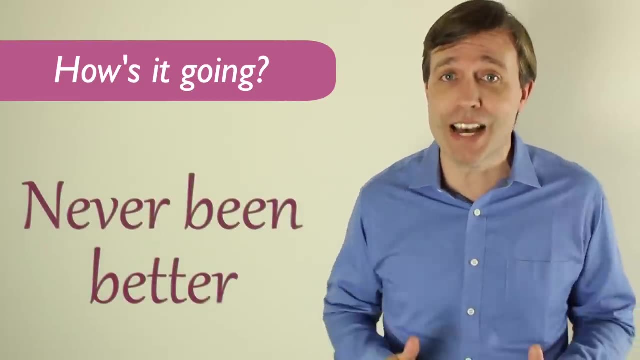 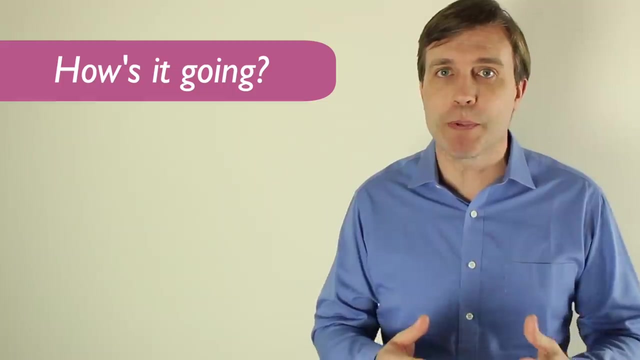 day, or even life in general, How's it going? And instead of saying good, you can say, yeah, great, fantastic, I'm doing well. Or you could even say: never been better, If you think that you're just very good. Now, if you want to express that well, that you're good but not really show a whole lot. 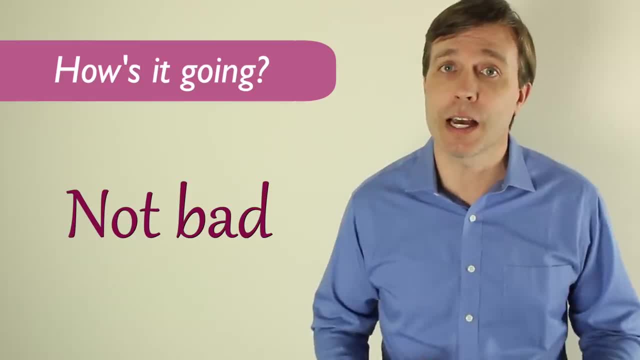 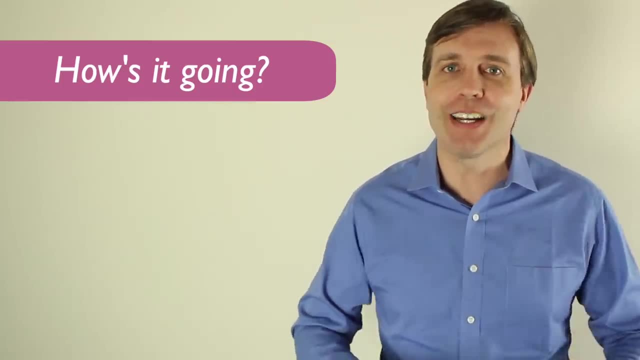 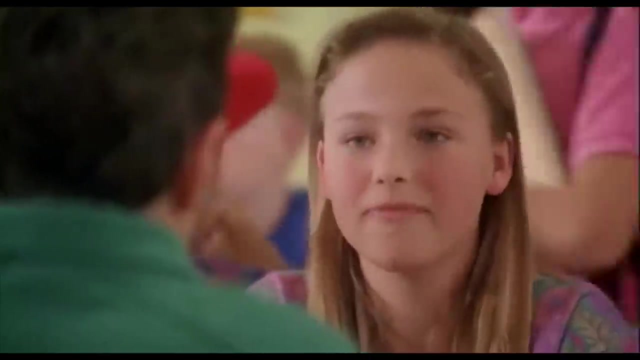 of enthusiasm. then you could just say: well, not bad, I like to use that one: How's it going, Not bad? Or you could even just say okay, which is another very common word, but you could use it instead of good: Hi, Hey, how's it going Okay? Hi, Tiffany, Hi, Roger, How's it going, Not bad? 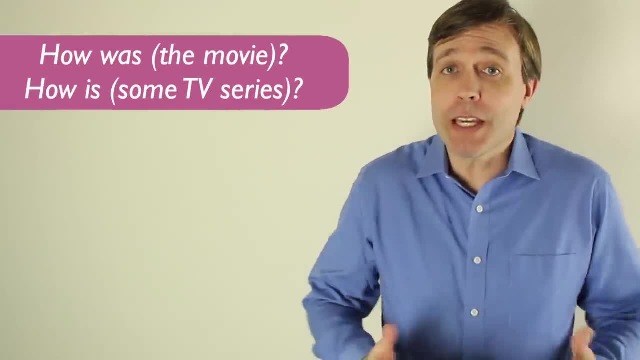 Then we have a very common question: How's it going? Not bad, How's it going Not bad, Not bad. Then we have the question: how was the movie? Or maybe even somebody could ask you: oh, how's this? 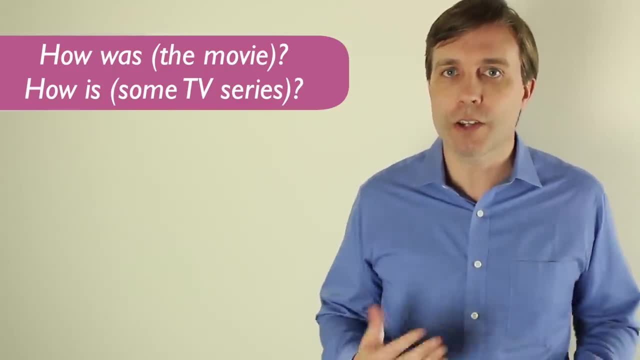 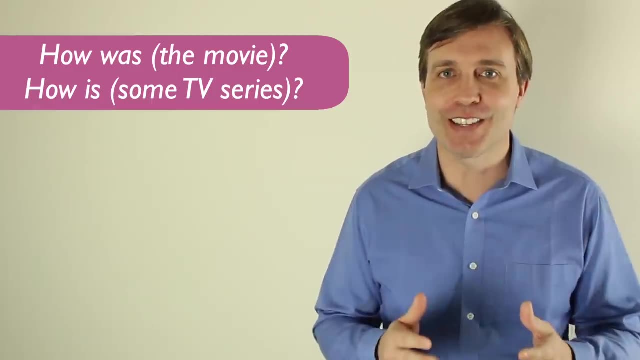 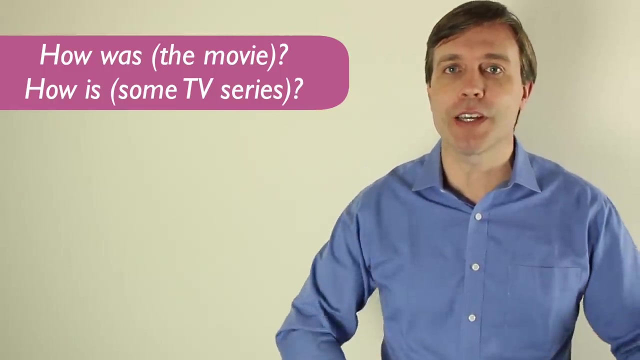 TV series. These are common questions because we like to talk about movies and TV, And I would always get this whenever I'd ask students: well, how was the movie Good, good, good. So instead of saying good, you can say that well, it was spectacular Or it was a must see. If it's a must. 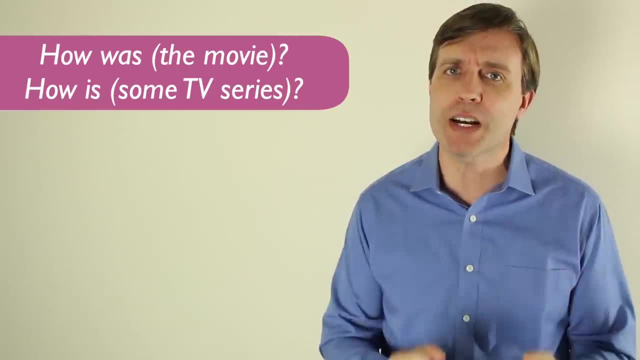 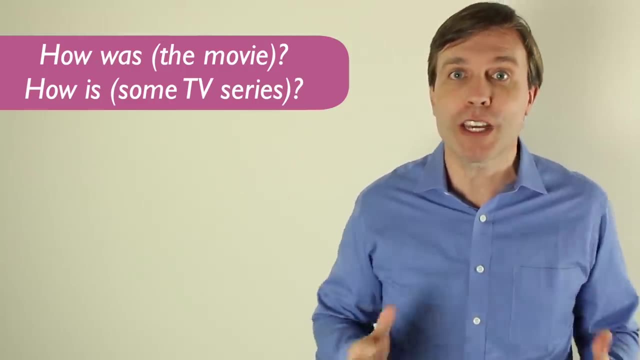 see. really, you have to see it. But it's a great way to describe a movie as a must see. Or maybe you could say it was entertaining, fascinating or captivating- Those are some great adjectives. Or even riveting, That's another. that's another good word, If, if something keeps you on the edge of 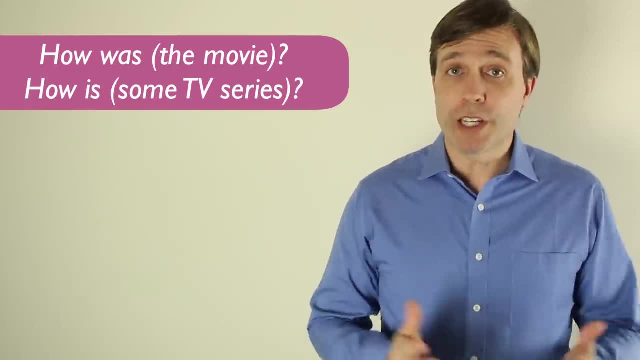 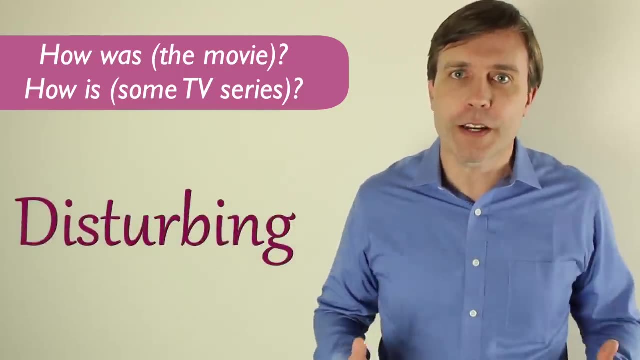 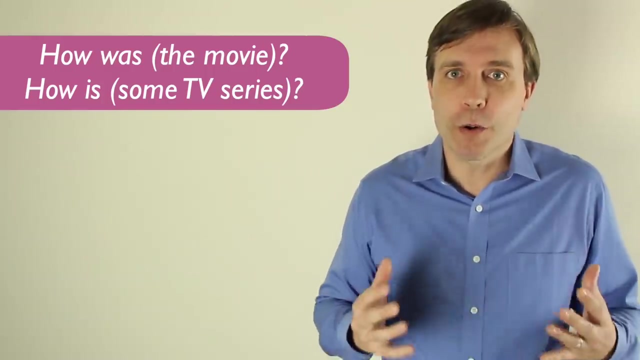 your seat you could say, wow, it was riveting. Or if the movie or TV show is funny, you could say it was hilarious. Or if it's scary, it was frightening or disturbing, Or even it was powerful. It really it. it affected me. It was a powerful movie, Or maybe it was something it made you think. 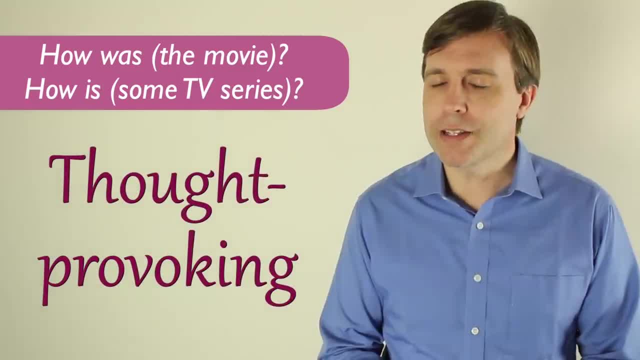 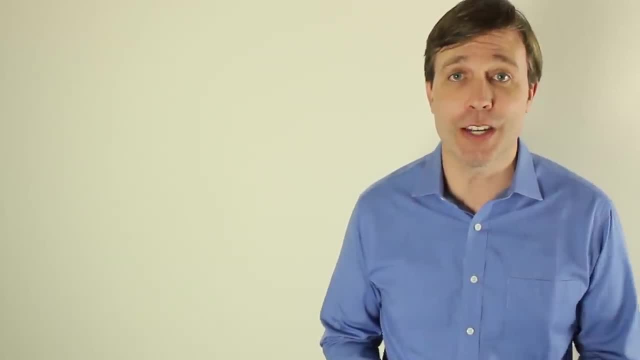 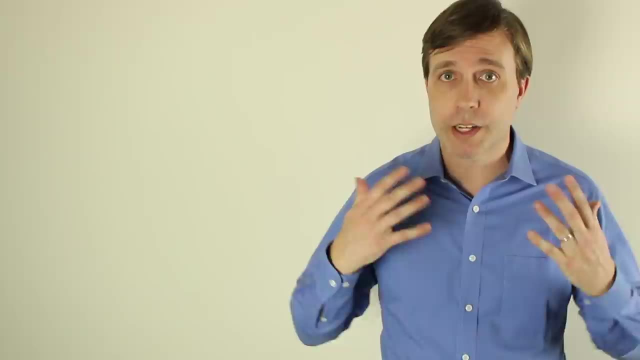 you could say it was. it was thought provoking That TV show. it was thought provoking- That's another great adjective that you can use instead of saying: good Documentary now has presented audiences with the world's most thought provoking cinema. Now, if you want to start expressing, 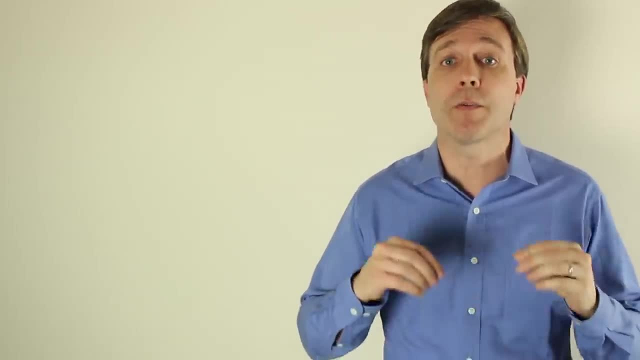 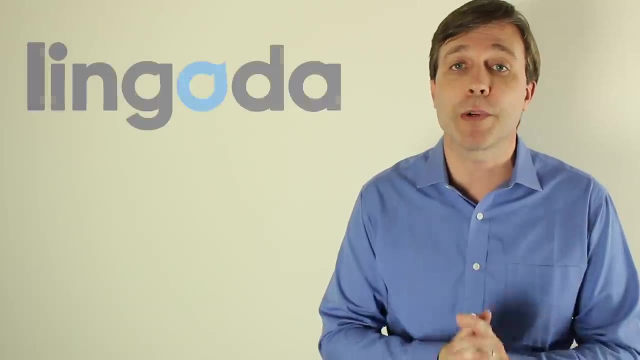 yourself using many different adjectives, like the ones that we're learning in today's lesson, then you just need to practice, And a great way to get practice is by taking some online classes with Lingoda, who is the sponsor of today's lesson. And if you want fluency success, then I 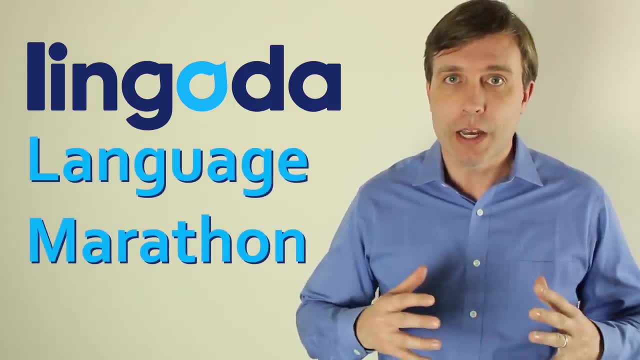 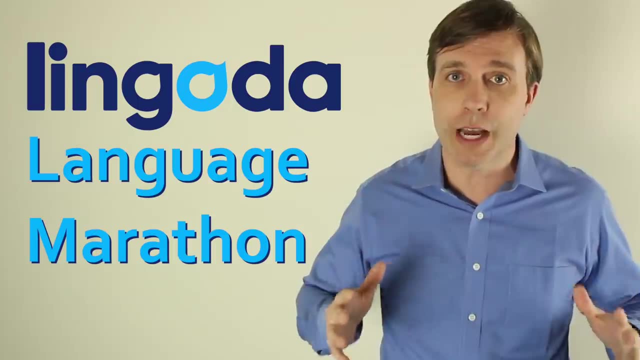 recommend you check out the Lingoda language marathon, because learning a language is like training for a marathon. If you are learning over a longer period of time, that is just going to help you continuously improve your skills, And there are three different options for the Lingoda. 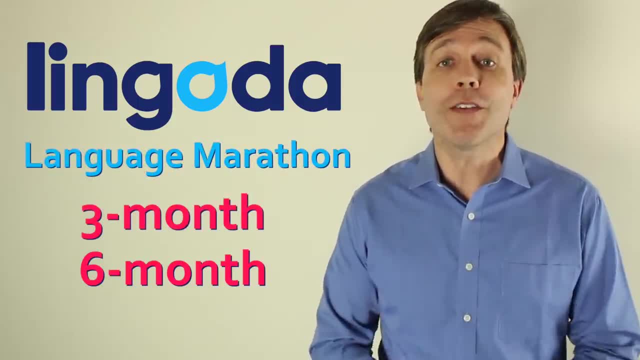 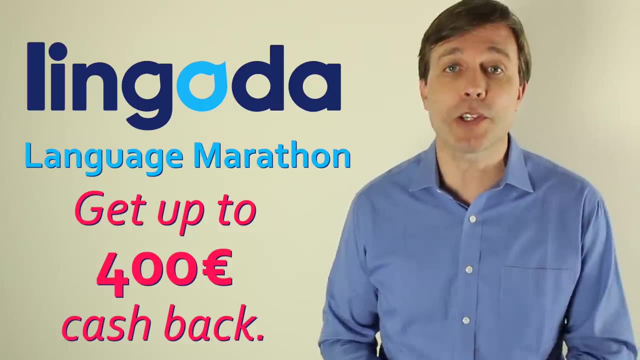 marathon challenge. You can take the three-day marathon challenge, which is a three-day marathon challenge- the three-month, the six-month or even the 12-month marathon- And you can also get up to €400 cash back if you attend 90% or more of the lessons during the marathon. 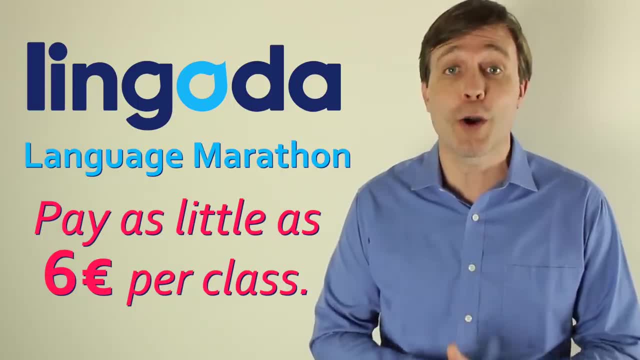 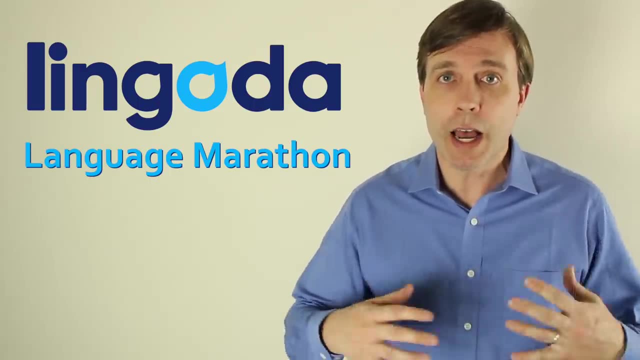 period, which means that you could pay as little as €6 per class. The reason this will really help you is because you will have small group classes with a native speaking teacher, And I know this because I took some Spanish classes with Lingoda and I had a lot of opportunities. 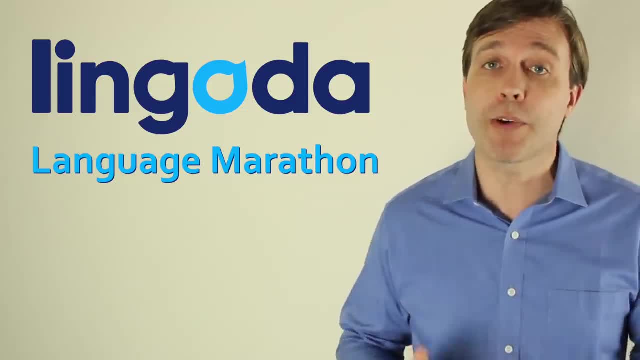 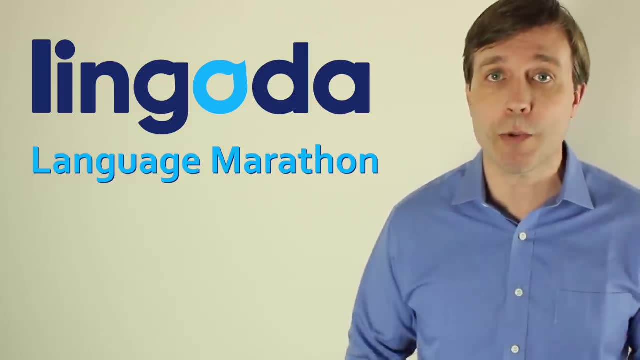 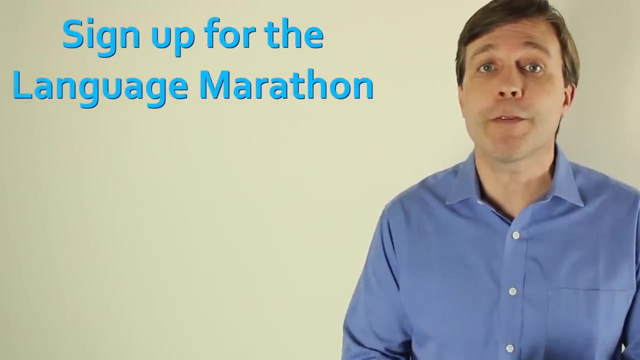 to speak. I was able to learn new vocabulary And actually practice using the grammar in conversation. You will also have the flexibility to take classes anytime, anywhere. Just click on the link in the description if you want to give the marathon a try, And you have two choices. You can take a seven-day free trial. 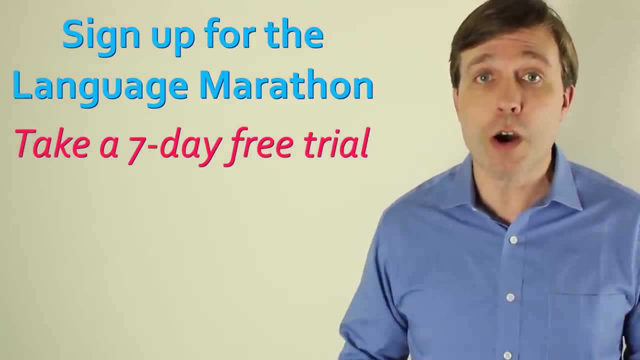 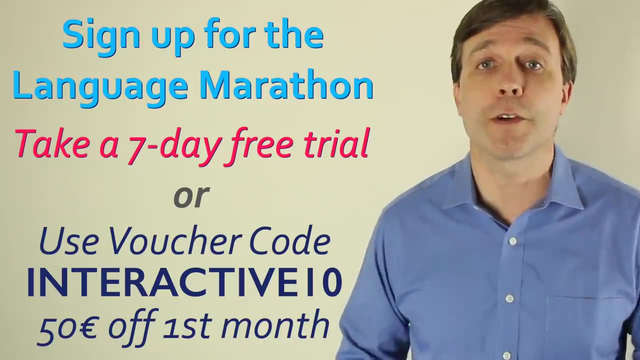 if you want to see if the marathon is right for you, Or if you know that you want to sign up for the language marathon, then you can use the voucher code INTERACTIV10 and get €50 off your first month. So click on the link in the description if you would like more. 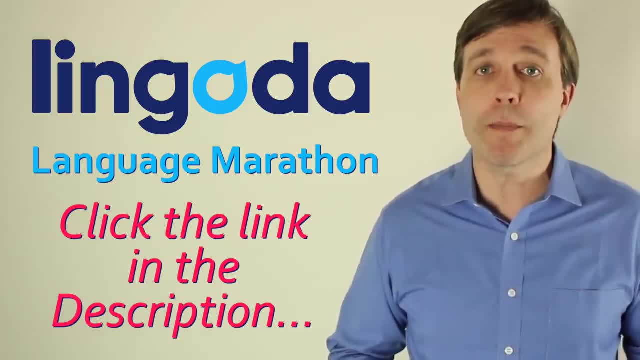 information about the language marathon and sign up if you want to make this your year for fluency success. And don't forget, use that voucher code, INTERACTIV10, to get €50 off your first month. So let's get back to our lesson on what you should say instead of saying good And another. 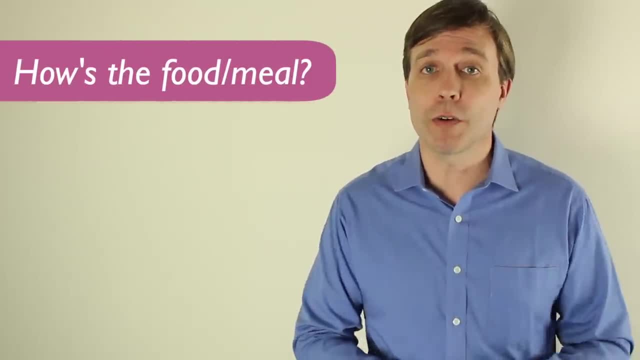 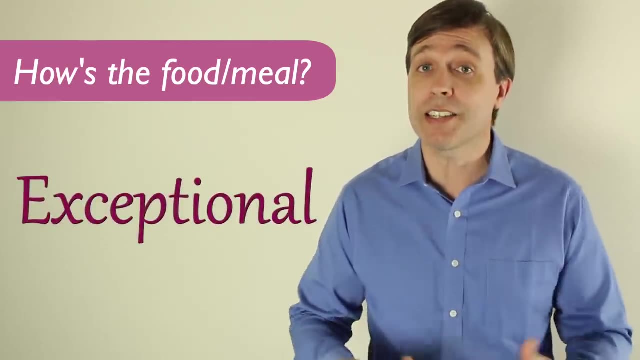 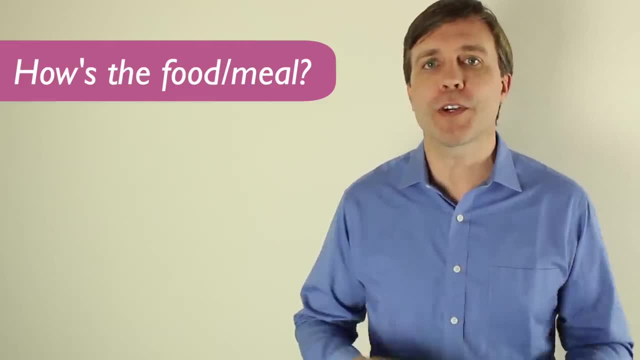 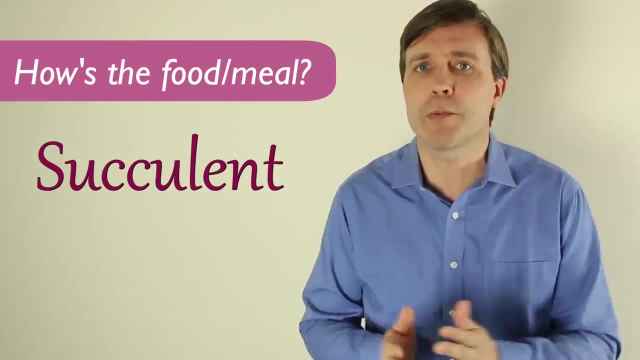 it. That's another very common response, But let's get a little more specific, And you could say that it is succulent. It means that something's delicious and also a little juicy as well. Another phrase that you could use to mean the same thing is mouthwatering. 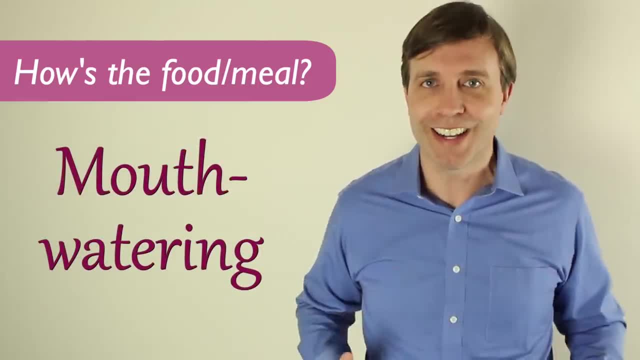 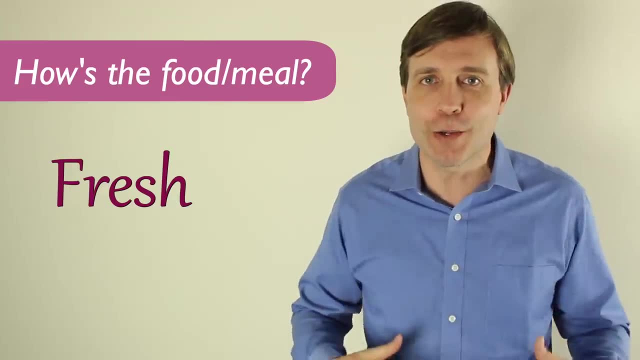 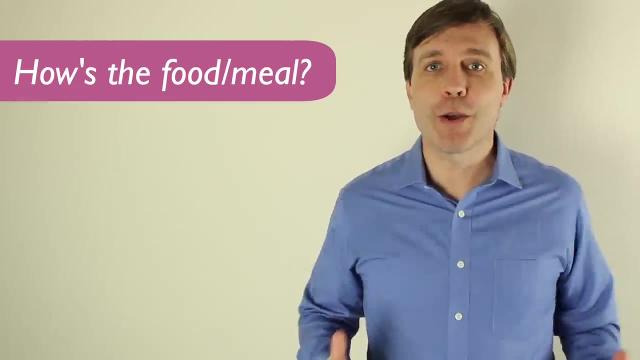 Oh, it's so good, It's mouthwatering. Or you could even say that something is fresh. That is a great word that I like to use, especially if I want to describe fruits, vegetables or bread, And I could say: oh, this is so fresh Now. those are all very positive ways. 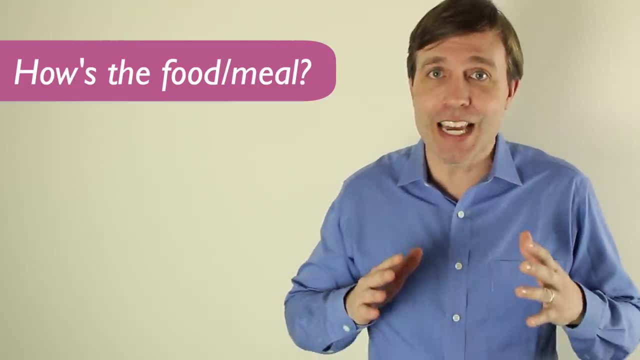 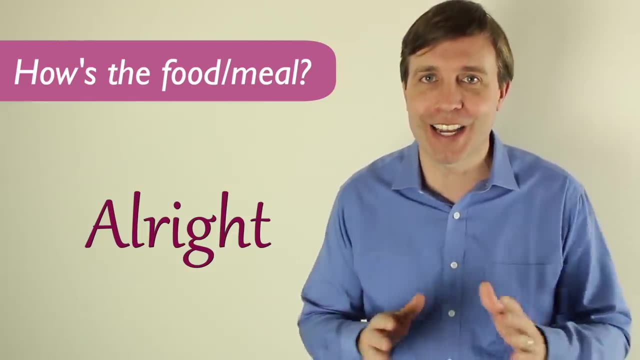 to describe food, And if you don't want to be so positive, then you could just say: all right, I, I, I'm guilty. I use this one quite often. It's a very common word And somebody says, oh, how's your food? And I say, yeah, all right, It's, it's good, It's all right. 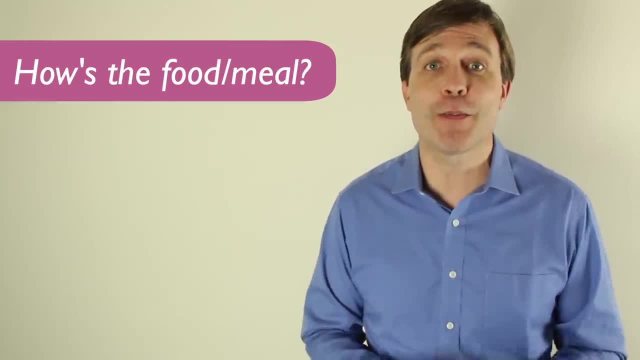 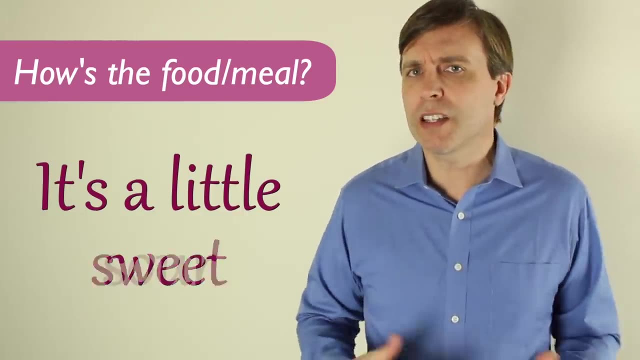 Or if you want to be a little more specific and give that extra bit of information, then you could say it's a little and then fill in any adjective: It's a little sweet, It's a little sour, It's a little spicy, It's a little bitter. 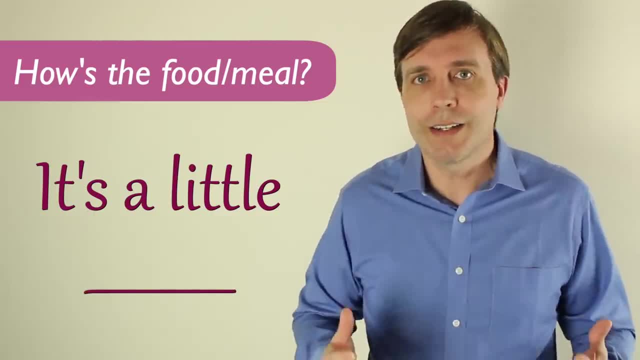 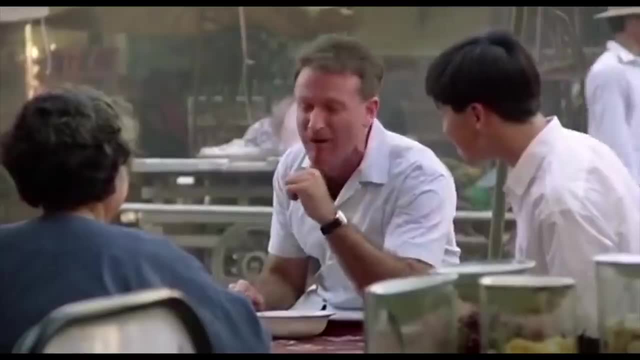 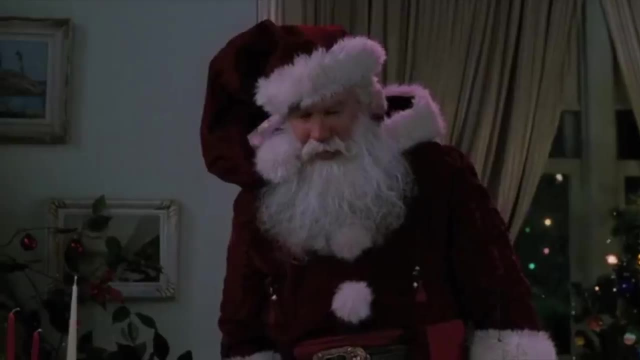 And this. this tells somebody that the food is good, but you know it could be better because, well, it's a little sweet, It's a little sour, It's a little bitter, It's a little. I think the milk's a little sour. It's soy milk. Here you go. They're a little spicy. 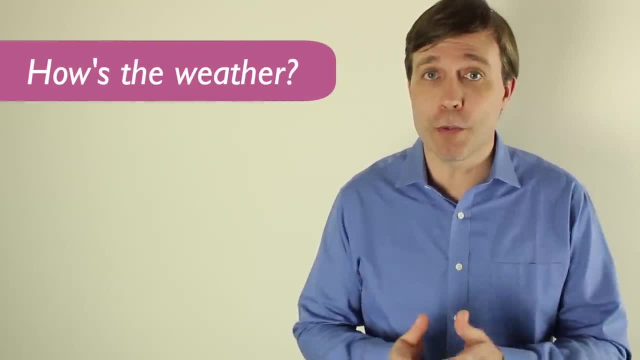 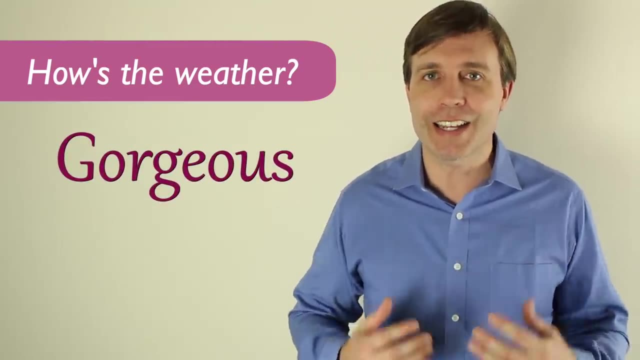 Another question that you could get is: how's the weather? And if you want to describe the weather, you could say: it's gorgeous outside. I love using that adjective to describe the weather And I say that quite often. Wow, You know it's. 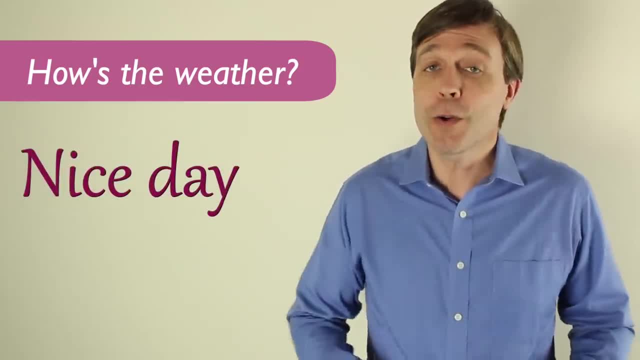 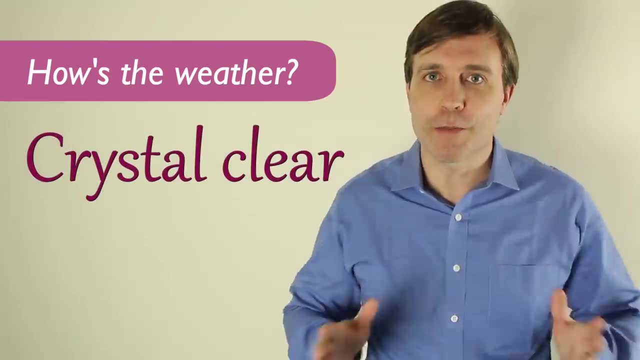 gorgeous outside. Or you could just say it's a nice day, or even it's a pleasant day, Or, if you want to give more information, you could say it's crystal clear. So if you say it's crystal clear, then typically there are no clouds in the sky, It's blue skies, all. 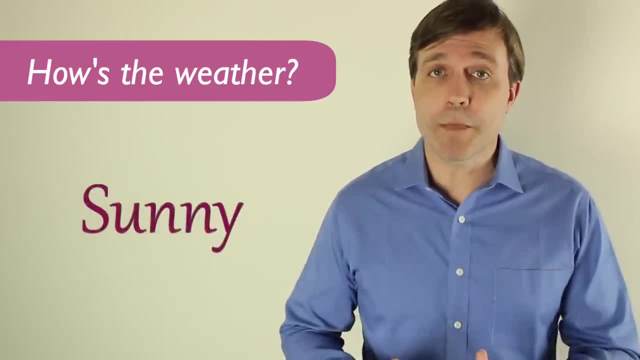 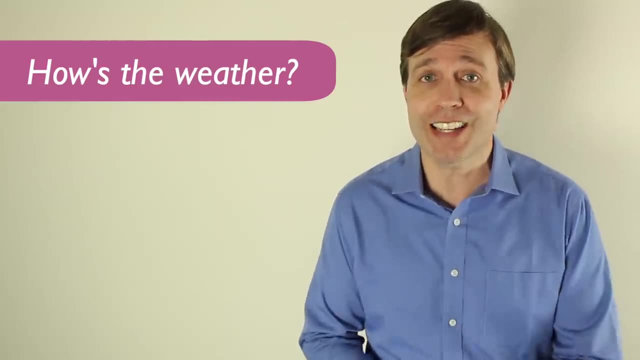 around. It's crystal clear. You can also say that it's sunny. I think people associate good weather with sunny weather and say, Oh, wow, it's a it's a sunny day. or even combine it with nice and say, wow, it's nice and sunny outside. You could. 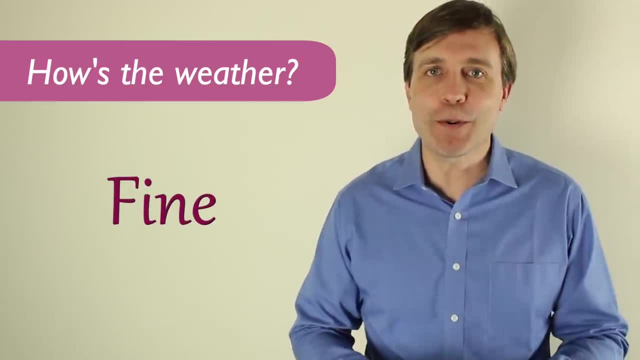 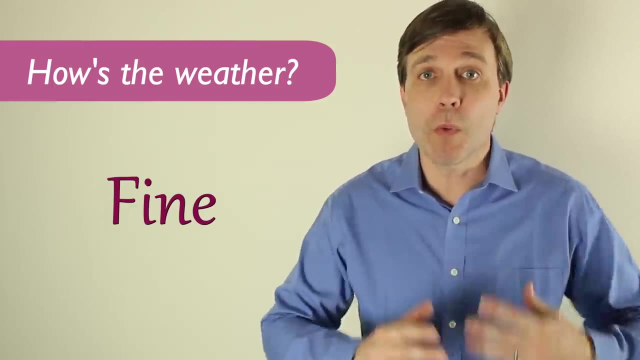 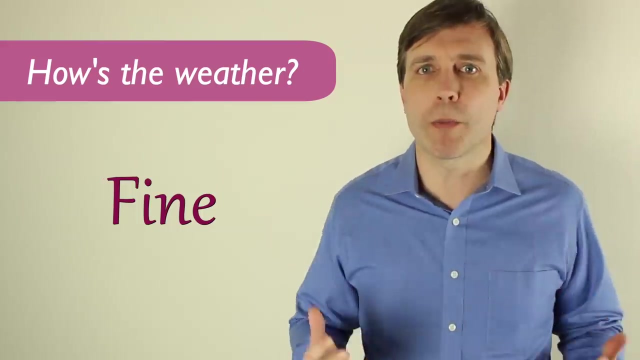 also say fine, And I think people would would just use this word if they're responding to the question and somebody is asking: well, what's the weather like, What should I expect when I go outside? And if you say fine, then it's more like: well, you know, it's normal. 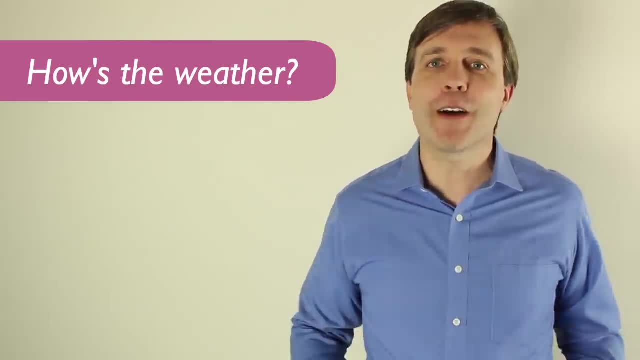 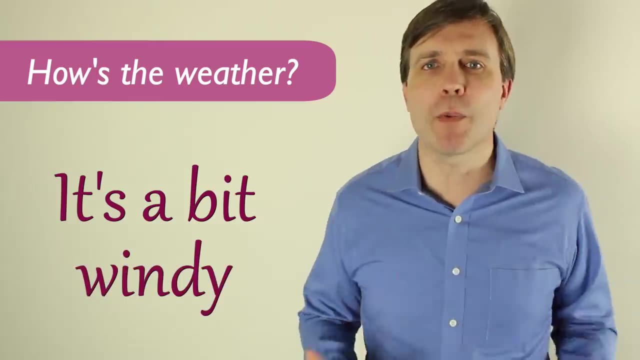 There's nothing strange, There's nothing unusual, It's, it's just fine. And finally, you could be more specific and say it's a bit, and then fill in whatever adjective: It's a bit windy, It's a bit cool, It's a bit chilly out, And. 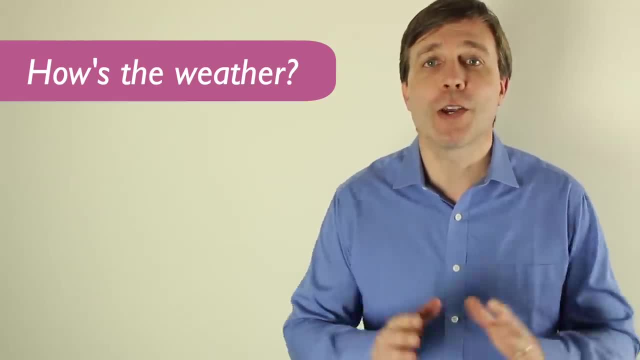 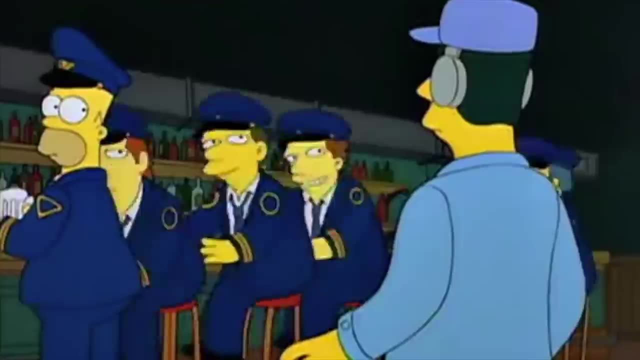 again that that just gives people more information So they know exactly what you're talking about. It's just a bit chilly in here, Don't you think We need a pilot city? Oh, I'll go. Conditions are a little windy. 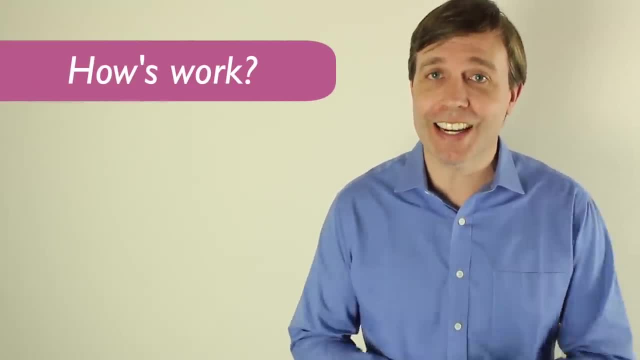 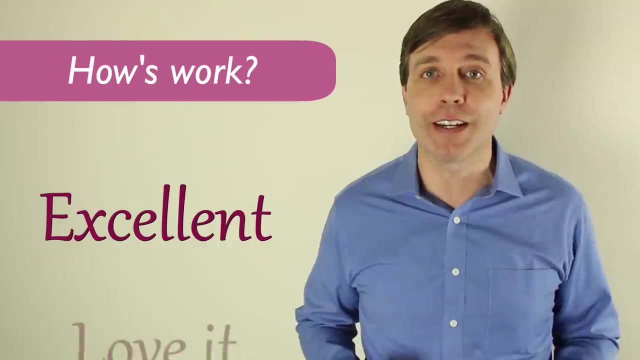 Another common question is why? Well, how's work going? How's work, And in that case they're talking about your job. So you could say that that it's wonderful, It's excellent, Or you just say I love it. 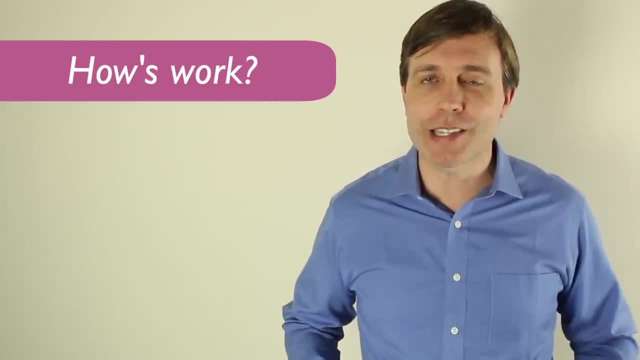 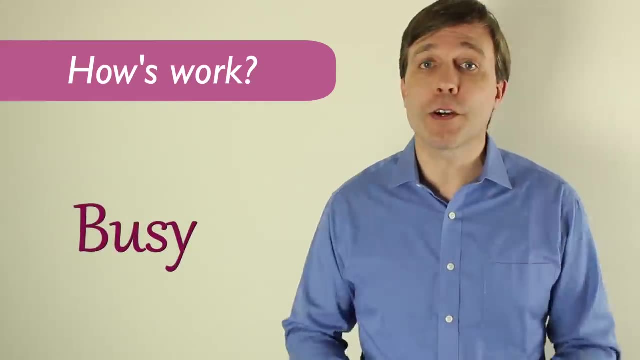 I love what I do. I love it. Or perhaps you could describe it and say that it is challenging, Maybe it's demanding, And if that's the case, you could also say that wow, it's. you know it's very busy. You could also say: I'm learning a lot of new things. I think this is a great. 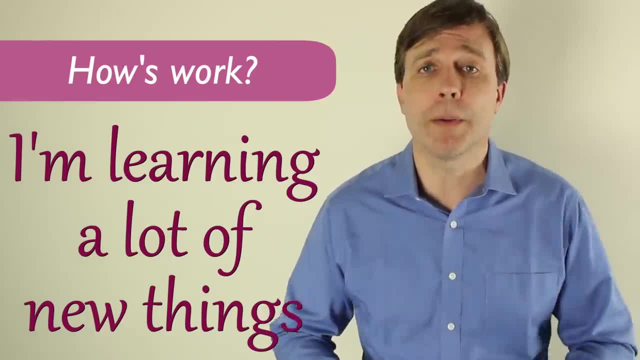 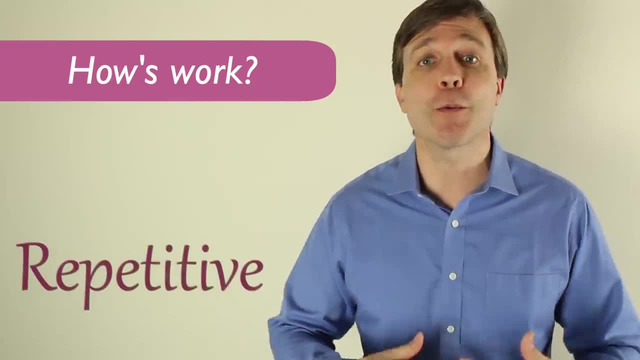 response, especially if someone just started a new job- I'm learning a lot of new things- Or if you've been working the same job for a long time, then you might say something like repetitive or even monotonous. How's work? Well, it's monotonous. I just do the same. 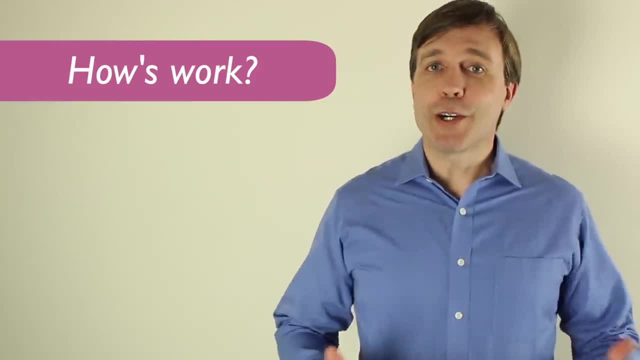 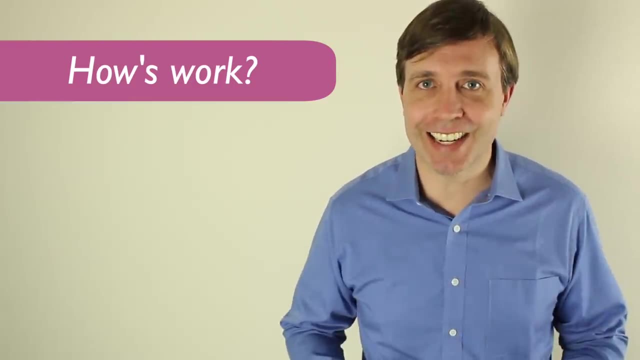 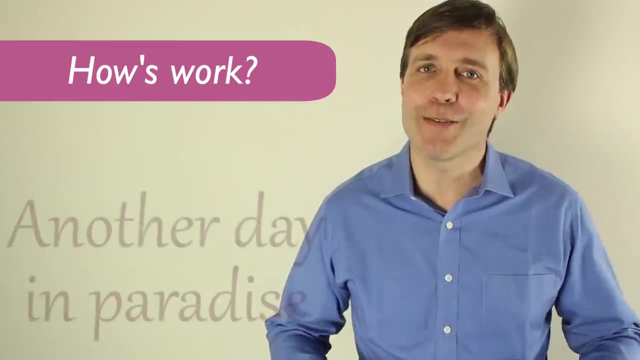 thing every day, day in, day out. It's monotonous. A job could also be lonely if you end up working by yourself all day, or if you want to be sarcastic and somebody says this and ask you this question- how's work going? And you don't really care for the work and you'd say: well, 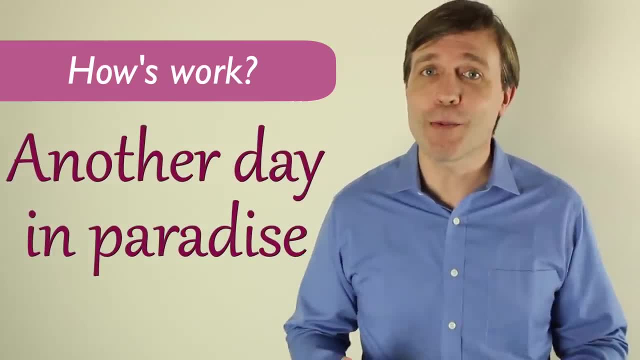 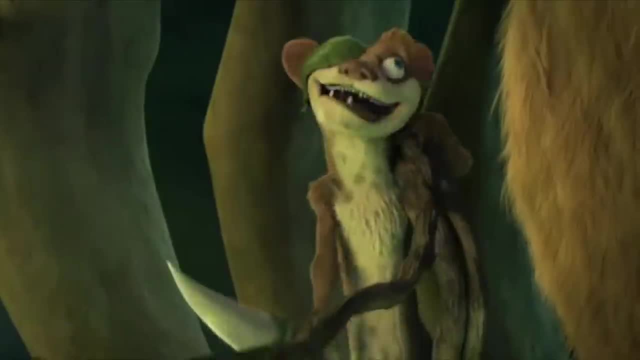 you know it's another day in business. Like you don't want to be all alone anymore, Like paradise. i don't really mean it, but that's a good way to express the way you feel about the job. read in the toxic fumes and you'll probably die toxic fumes. just another day in paradise now if 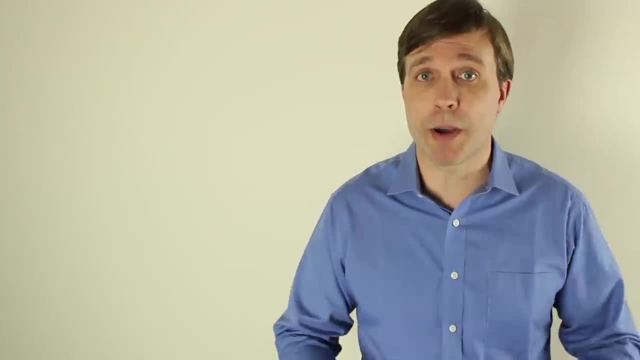 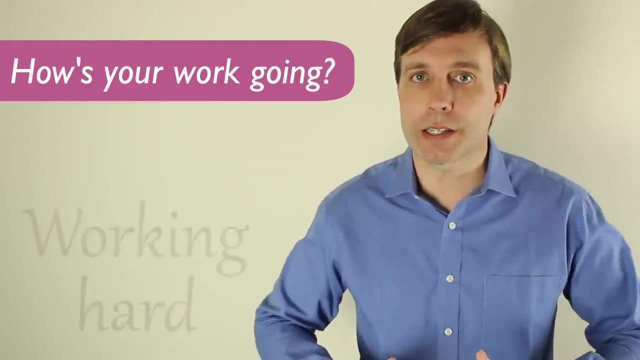 somebody's talking about some sort of project. when they ask about your work and actually the things that you're doing and they say, well, you know how's your work going, in that case, then you could say like something like, well, we're working hard. maybe you could say that, well thing, things are coming. 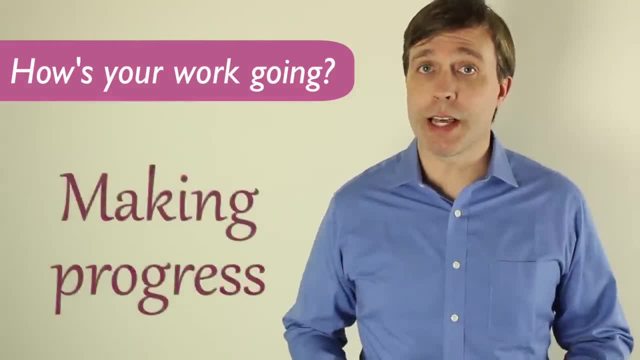 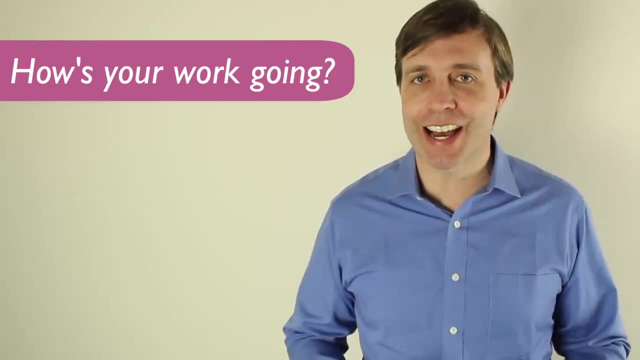 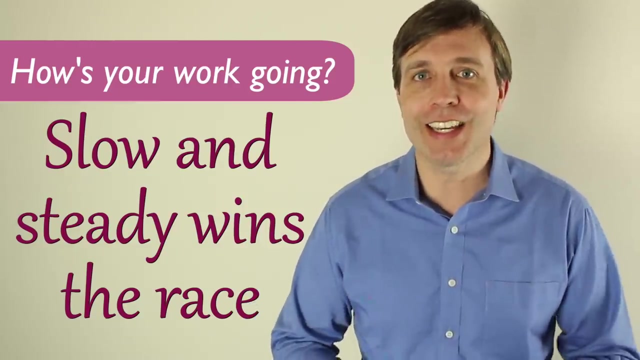 along nicely, thing, things are coming along or making progress. that's another great phrase to describe how you're working on some project, or an expression that i i think is a good one. you could just tell someone: slow and steady wins the race that if you continuously work. but even though 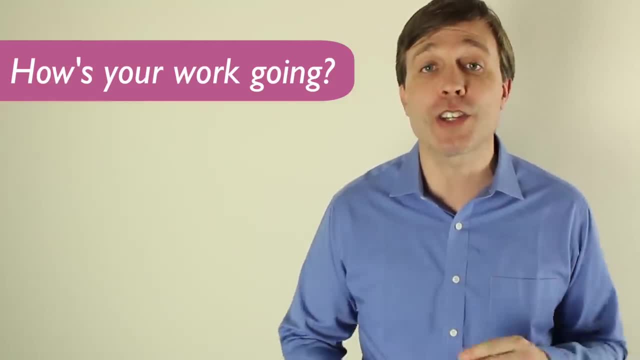 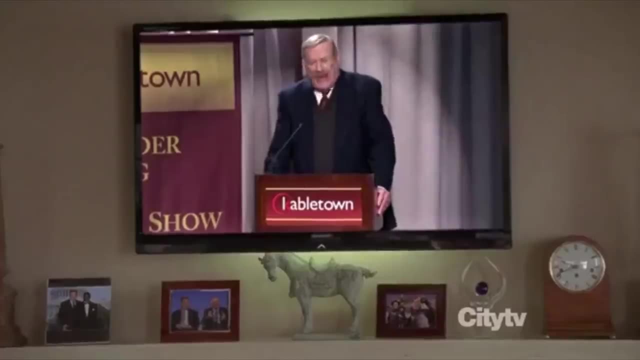 you're not going to be going very fast. slow and steady wins the race. you're still going to achieve your goal. chill out. slow and steady wins the race can't have you burning out. point is, i believe, that slow and steady wins the race. we don't take risks. we make profits. something else that people 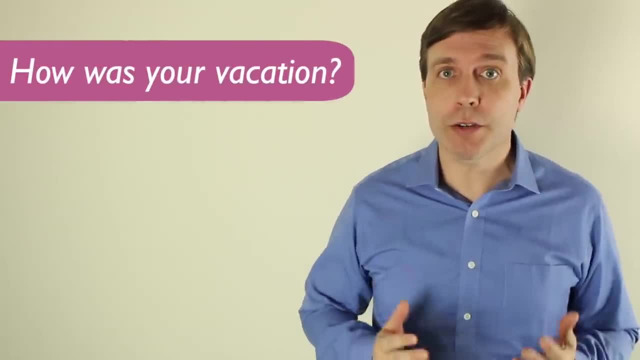 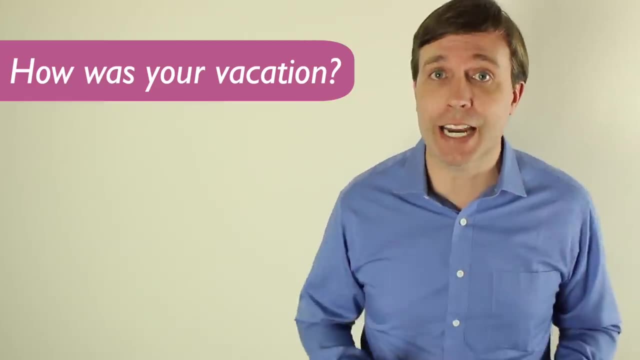 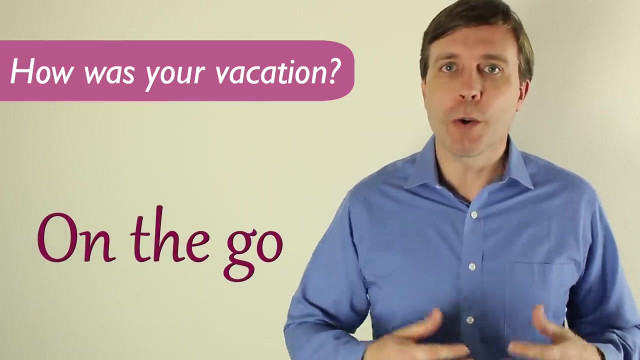 love to talk about is vacation. so somebody could ask you, you know how was your vacation, and there are different types of vacations. so if you, if it's, if it's very active, you could tell somebody maybe, well, it was adventurous. or perhaps you could say, you know, we were always on the go. or even you. 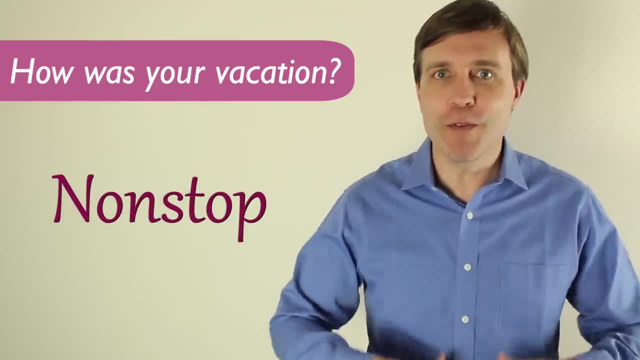 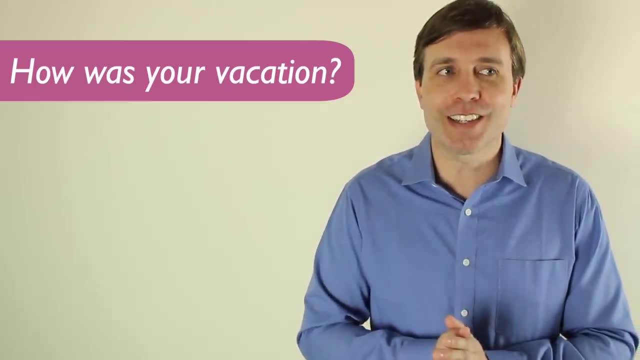 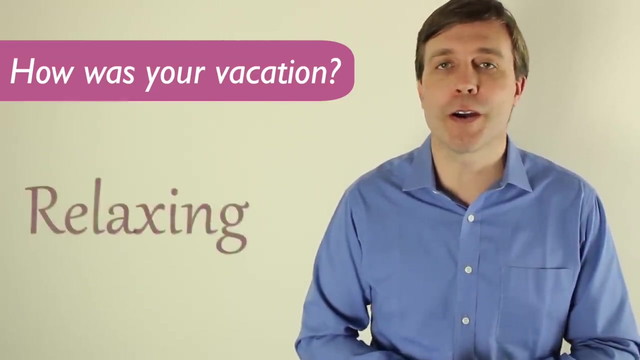 could use the word non-stop- that you were moving around, you were doing so many different things that well vacation it was non-stop. now other vacations are, are a little more calm, and in that case you might want to describe it as well. it was just, it was very relaxing. or perhaps you could say: 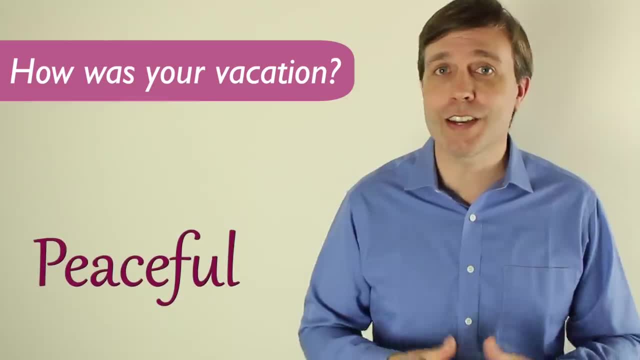 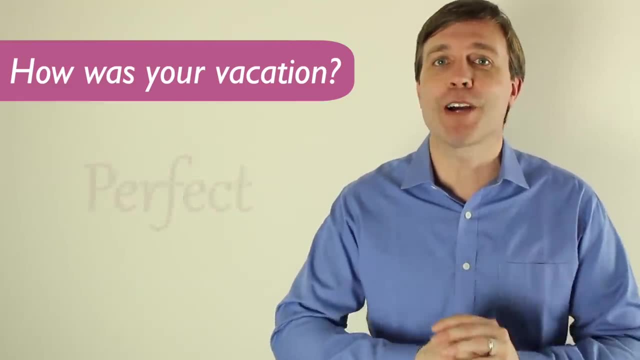 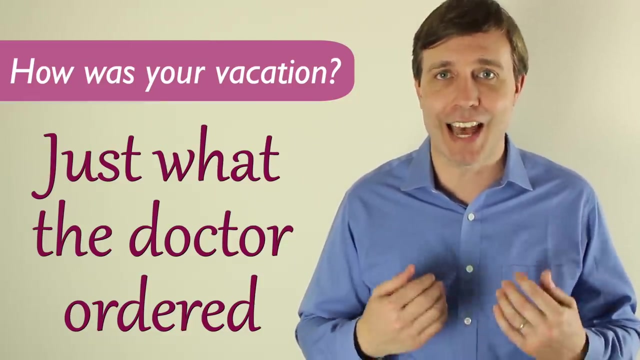 it was restful or maybe peaceful. that's another great adjective. if you absolutely loved your vacation, then you could say: it was perfect. or maybe a great expression is: it was just what the doctor ordered. this is an expression that means well they, you, you really needed to have this vacation, you needed this thing, and in that case you could tell: 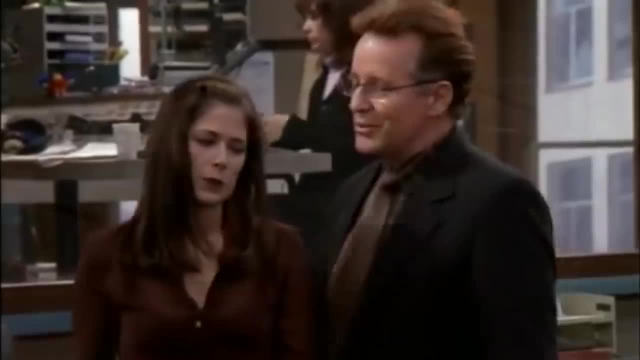 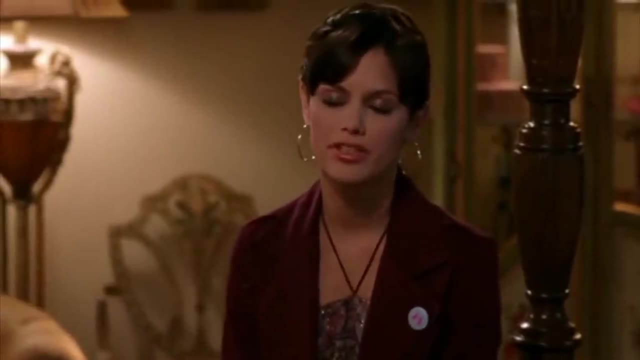 someone. it was just what the doctor ordered. a visit to the park was just what the doctor ordered. thanks, i was thinking, after the past few days you've had some pancakes on the pier and some serious sunbathing could be just what the doctor ordered. and if we're talking about an activity, 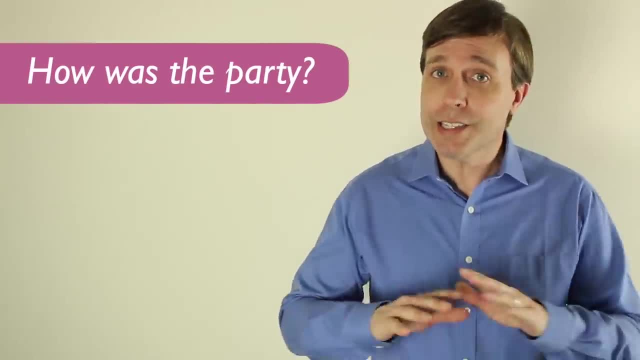 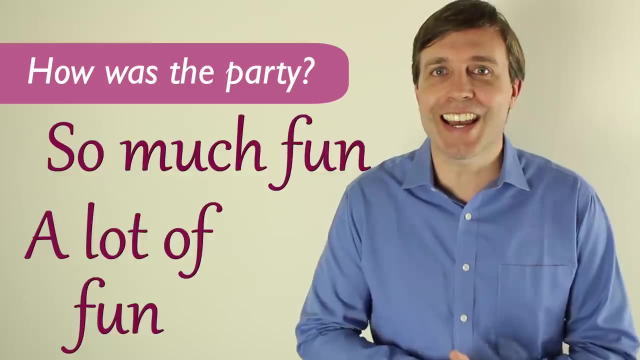 somebody could ask you a question like well, how was the party? and instead of saying good, you could tell them it was so much fun, or it was a lot of fun, or you could say it was off the hook. that is an informal expression, kind of an idiom or slang. 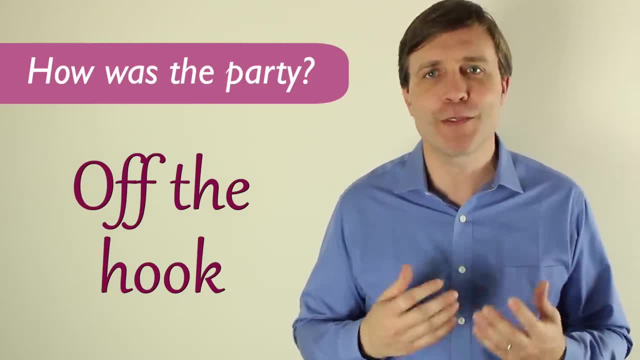 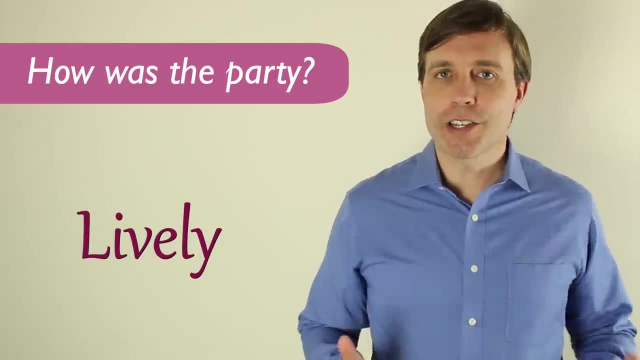 that means that it was well it was. it was a lot of fun. it was very cool that party. it was off the hook or maybe you would describe the party as lively. of course, not all parties are full of loud music and dancing. if we're talking about something maybe like a dinner party, you could 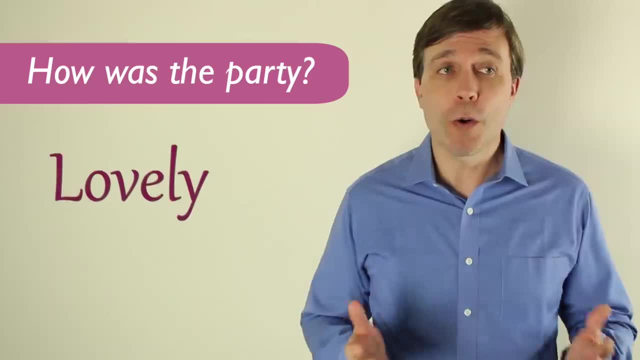 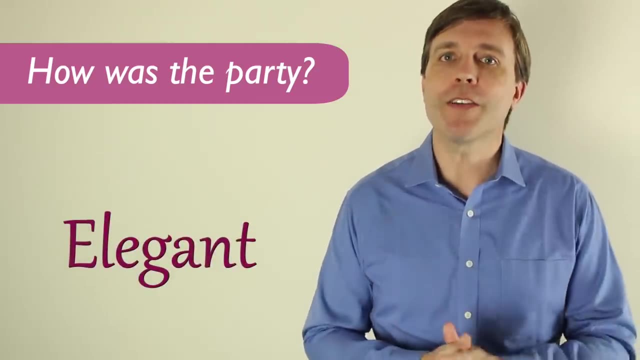 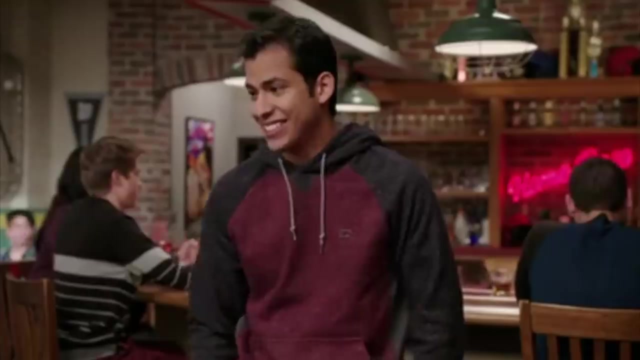 describe it and say, well, it was enjoyable or lovely. or, if you want to be more formal, you could say it was glamorous or elegant or even tasteful. those are some great adjectives to describe more of a. a formal party bought a great dress: burgundy, a-line, very tasteful. 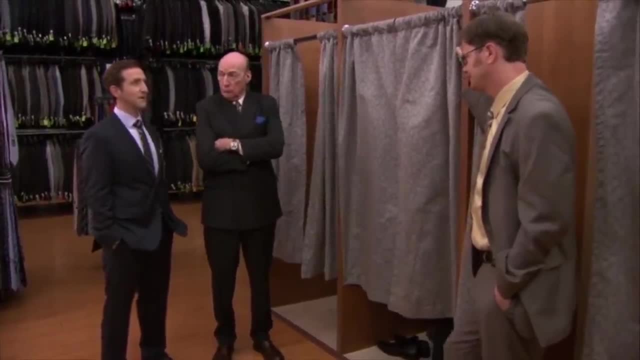 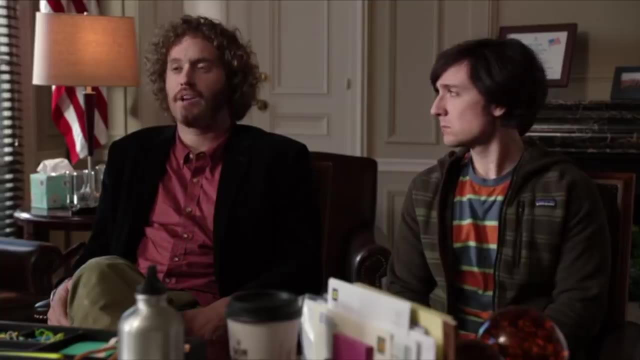 that's italian silk, very comfortable, very tasteful, although expensive. you just threw a million dollar party, a tasteful polynesian affair, culturally accurate. if we're talking about an event, somebody could ask: how was the party? and if you're talking about an event, you could say: well, it was a lot of fun. 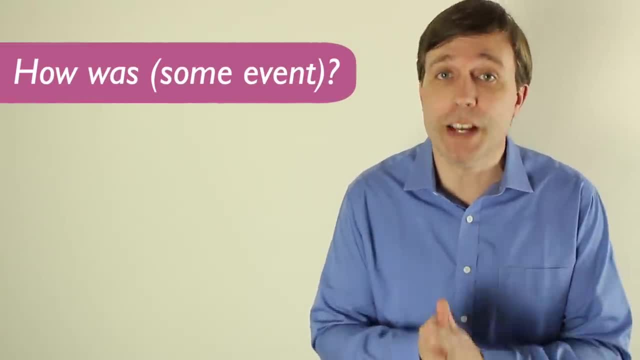 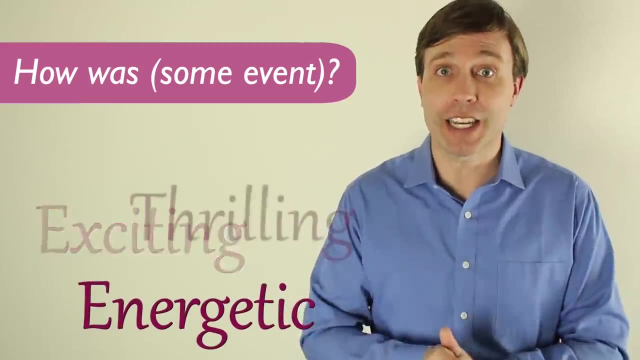 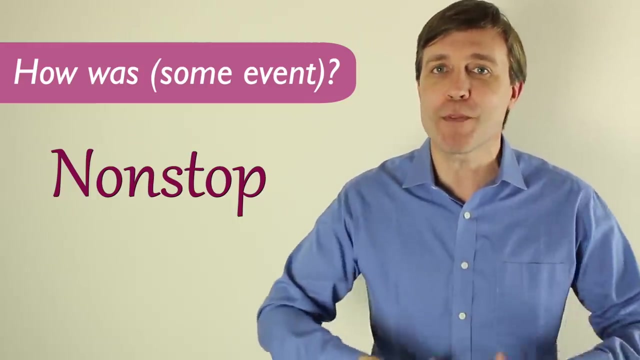 the, the football match, or how was the concert, or how was the festival? and instead of saying good, you can say: it was amazing, exciting, energetic, thrilling, marvelous or non-stop. now i told you i would not use the words and phrases more than once, so i'm going to. 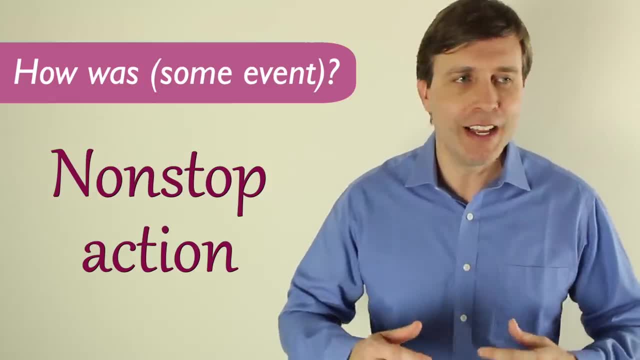 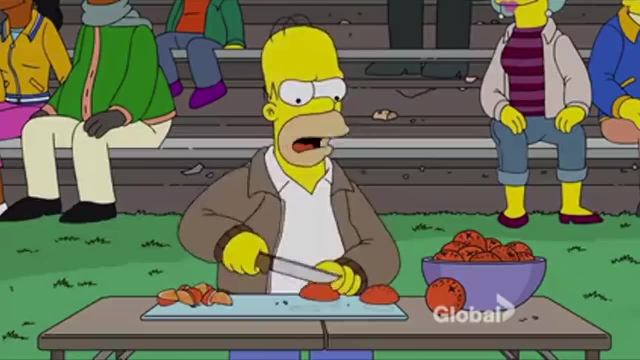 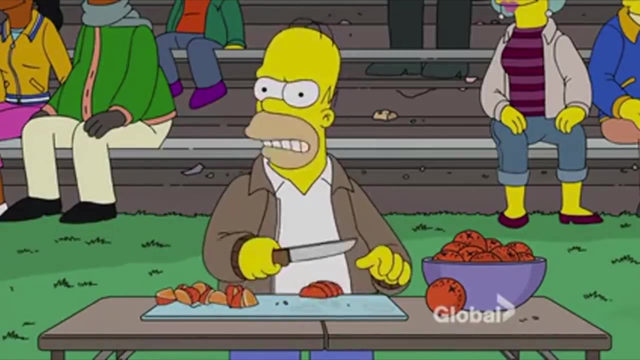 add another word and say non-stop action, that that things were just continuous and it just kept going. it was so exciting. you say, wow, it was just, it was non-stop action. i'm thrilled by the non-stop action kids running towards me with a look of joy i've never seen. 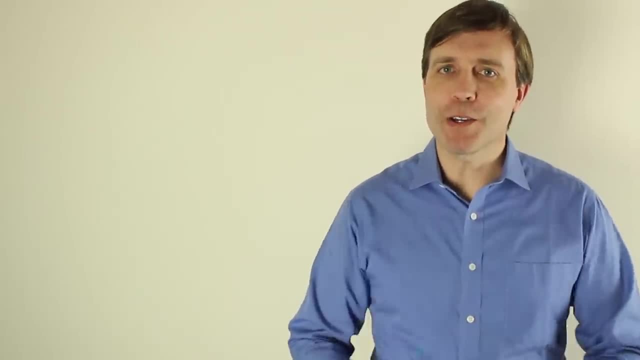 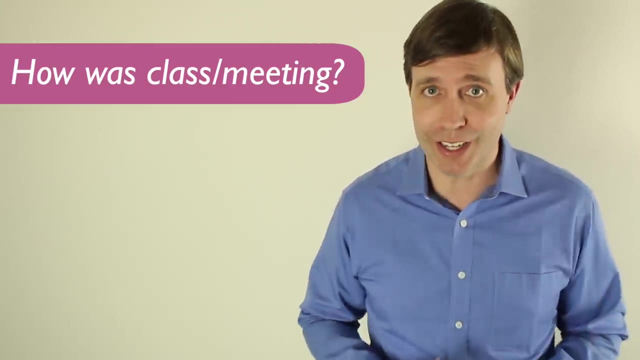 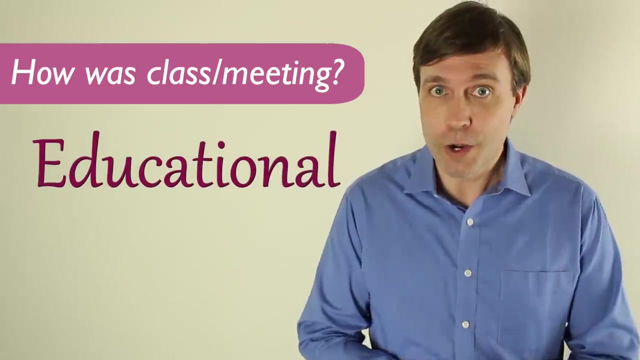 before and somebody might also ask you about your class or maybe a meeting, and they'll say: you know how was class or how was the meeting, and in that case don't use good. instead you could tell them that well, it was interesting or educational, or it was cool, very cool. you could also say: